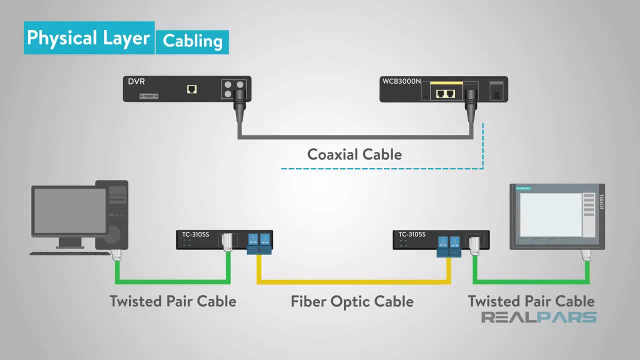 As stated previously, Ethernet cables come as coaxial cable which is not very common except in older installations, twisted pair, or intercontinental cables. 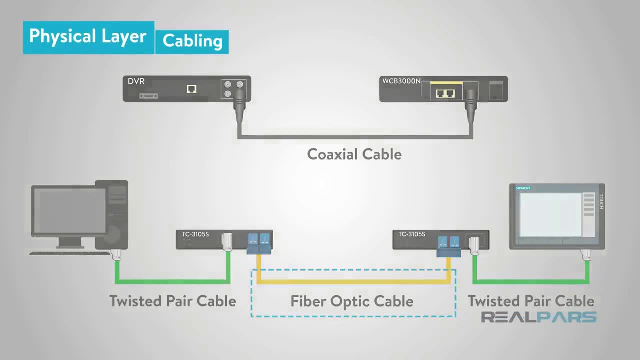 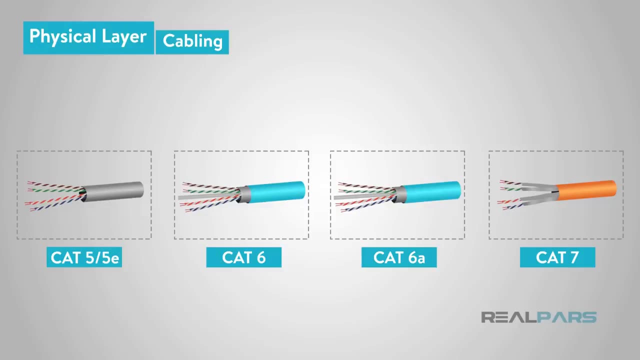 The most common cable is twisted pair cables, with the latest being Category 6 with speeds up to 1 gigabit per second 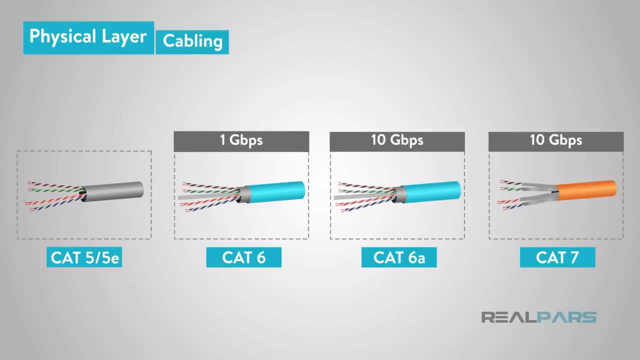 and Cat 6a and Cat 7 with speeds up to 10 gigabits per second. 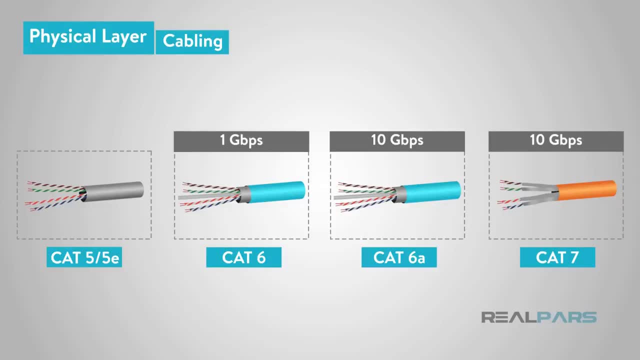 Category 5 and 5e cables are both still used in many existing applications, but handle the lower speeds between 10 megabits per second 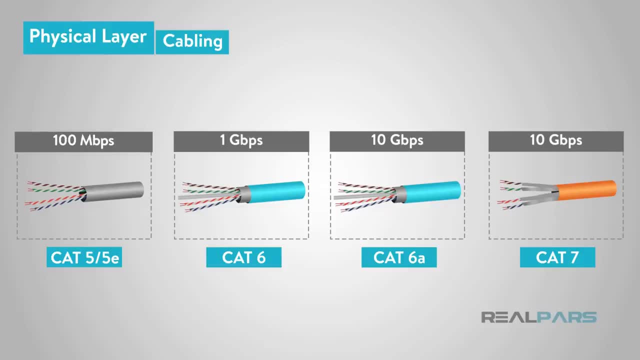 to 100 megabits per second, but are more susceptible to noise. 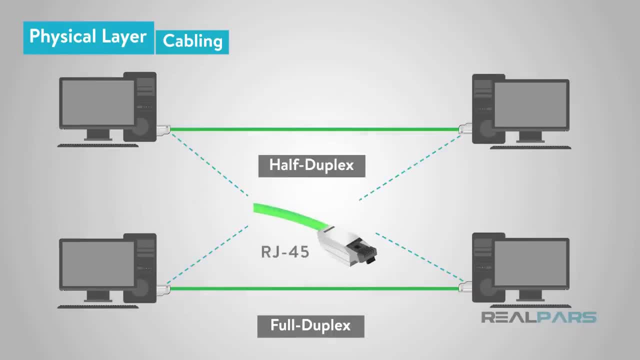 The Ethernet twisted pair utilizes RJ45 8-pin connectors at either end of the cable that is pinned for transmitting and receiving data in either half or full duplex mode. Half duplex transmits data in one direction at a time, while full duplex allows data to be transmitted in both directions at the same time. 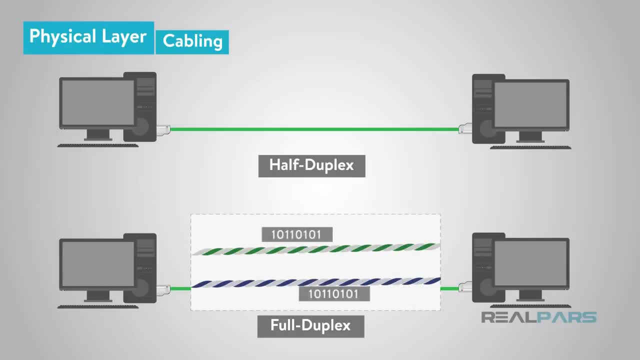 Full duplex in Ethernet can be achieved by using two pairs of wires to allow data to travel both directions simultaneously. 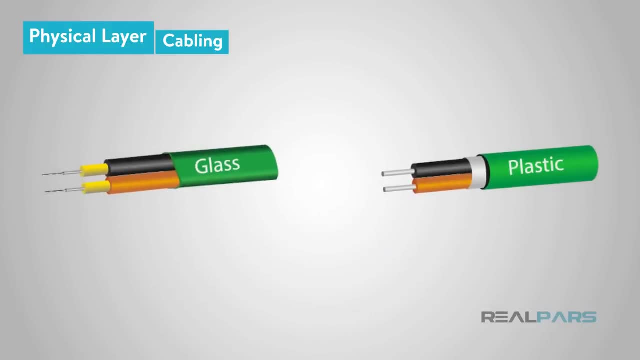 Fiber optic cable uses glass or plastic optical fiber as a conduit for light pulses to transmit data. 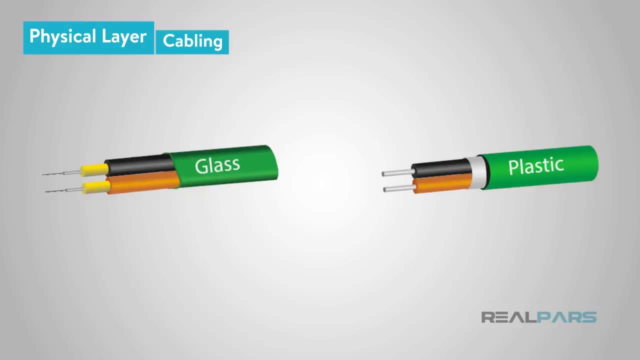 It has allowed Ethernet to travel farther distances at higher speeds. 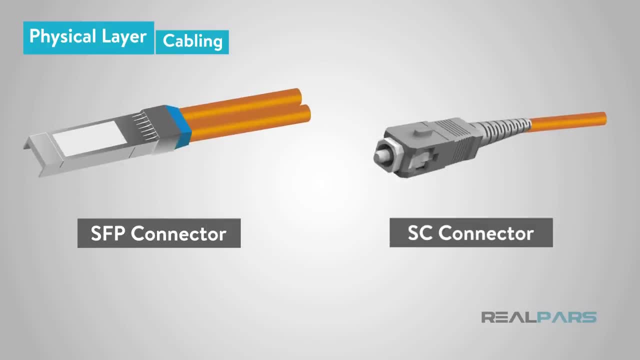 Fiber optic cables use several different types of connectors that vary depending on your application needs. Some of the different types are SFP and SC also known as square connector or standard connector. 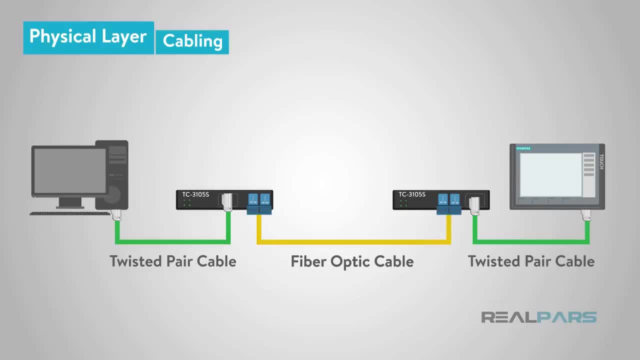 In order to use fiber optic in an Ethernet network that utilizes twisted pair Ethernet cables, you need to use an Ethernet to fiber converter that will allow your network to take advantage of the higher speeds of fiber optic and lengthen the distance that the Ethernet network can reach. 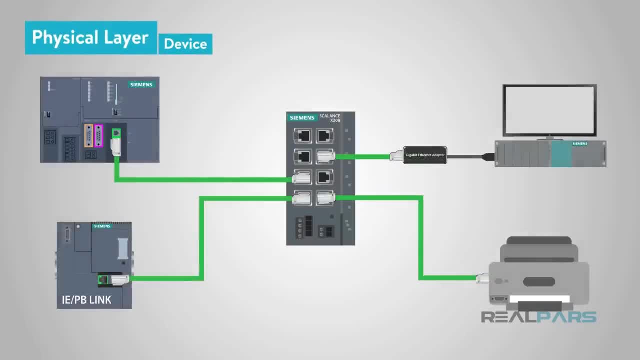 How about the Ethernet devices? Ethernet devices are consisting of computers, printers or any device 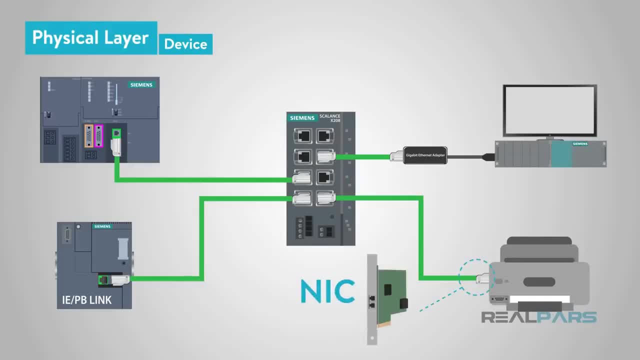 which either have an internal NIC or network interface card or an external one that is USB, or PCI based. 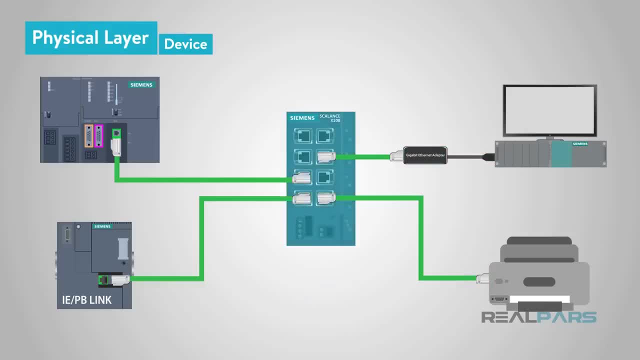 Switches and routers that act as the director of the network and connect multiple computers or even networks together to enable communication between all the different devices. 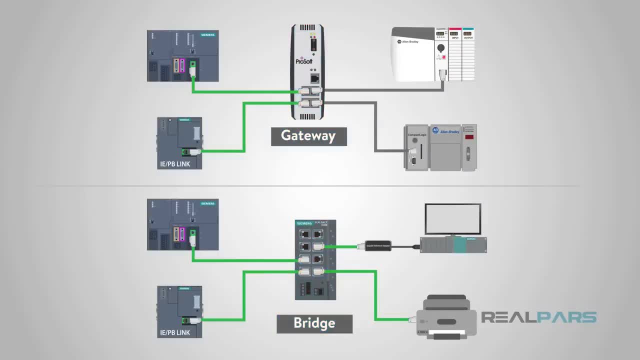 Gateways and bridges are used to connect multiple Ethernet networks together and allow communication across them. 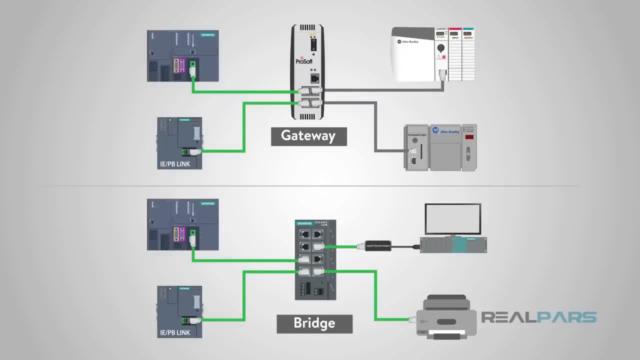 Gateways connect two dissimilar networks together while a bridge connects two similar networks together 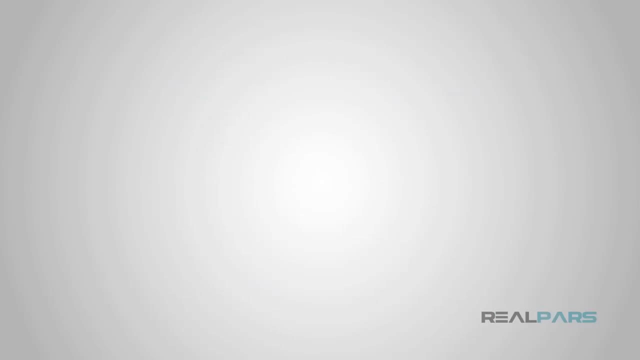 so that you can only see one network. 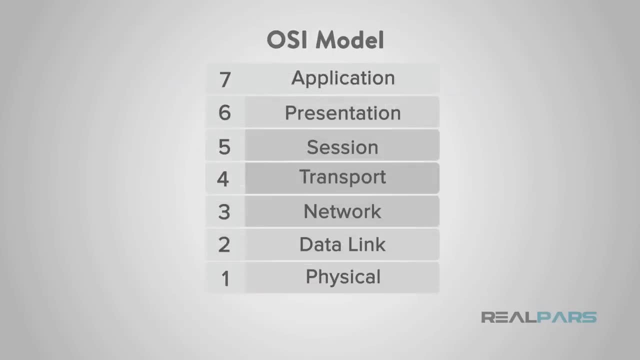 Now that we have discussed the basic physical components of Ethernet, let's move into the second layer of the OSI model, the data link layer. 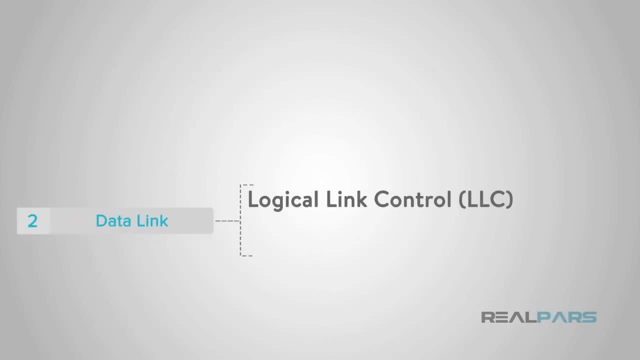 The data link layer can be split into two sections, the Logical Link Control or LLC and the Media Access Control or MAC. 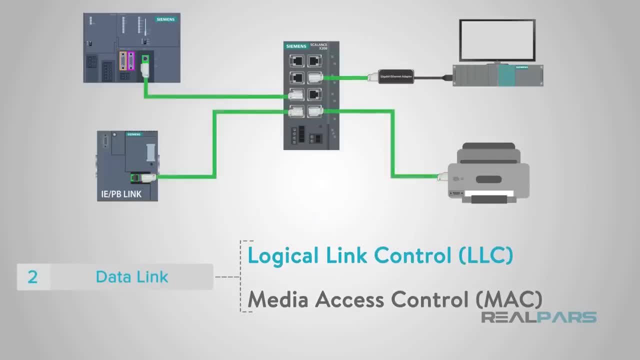 The Logical Link Control establishes paths for data on the Ethernet to transmit between devices. 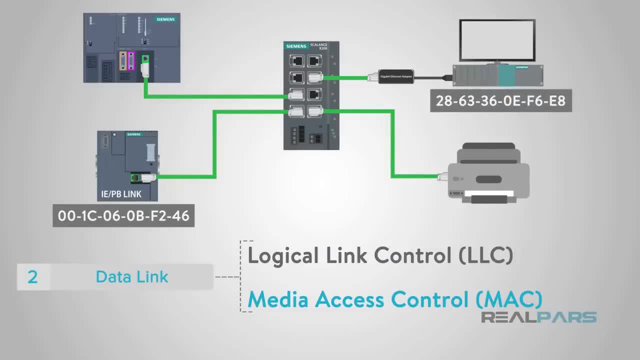 The Media Access Control uses hardware addresses that are assigned to network interface cards or NIC to identify a specific computer or device 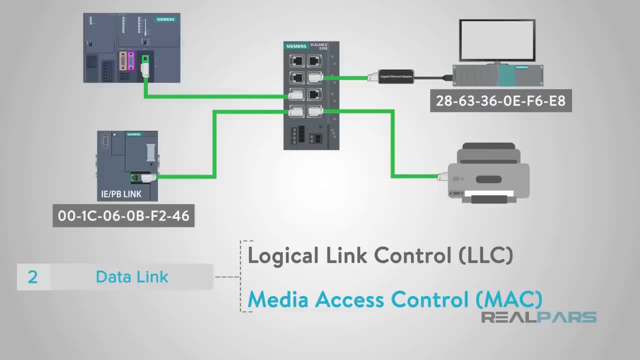 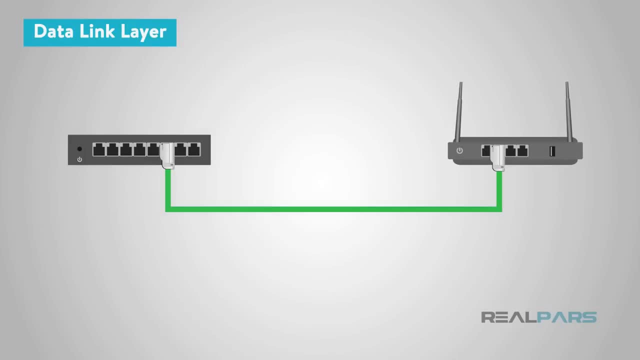 to show the source and destination of data transmissions. Ethernet transmits data packets in this data link layer by using an algorithm called 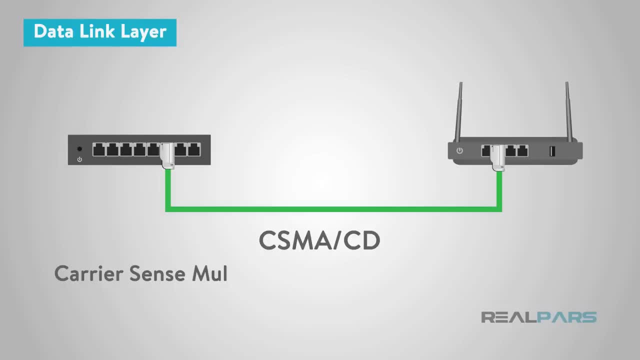 CSMA-CD or Carrier Sense Multiple Access with Collision Detection. 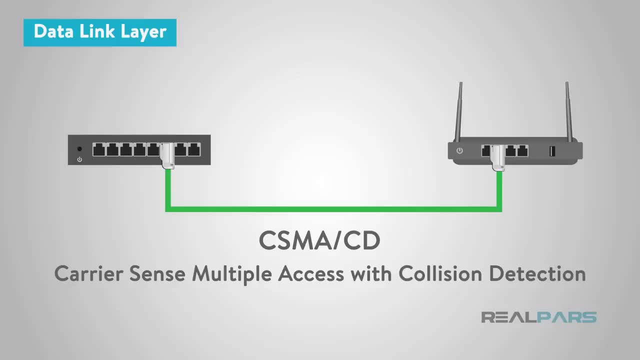 CSMA-CD is used as a standard for Ethernet to reduce data collisions and increase successful data transmission. 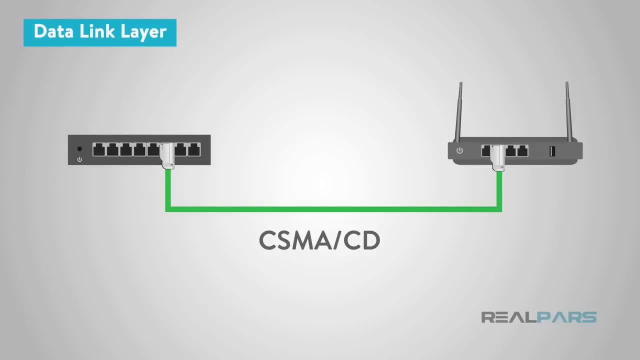 The algorithm first checks to see if there is traffic on the network. If it does not find any, it will send out the first bit of information to see if a collision will occur. If this first bit is successful, then it will send out the other bits while still testing for collisions. 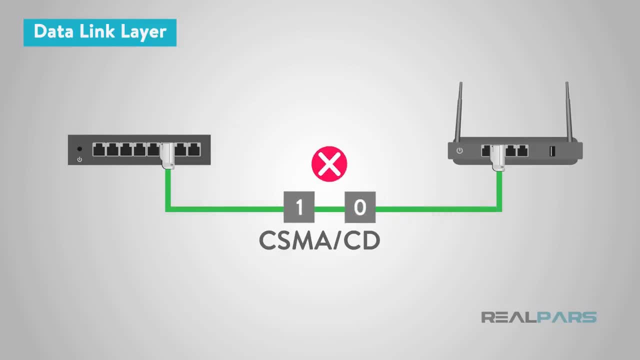 If a collision occurs, the algorithm calculates a waiting time and then starts the process all over again until the full transmission is complete. 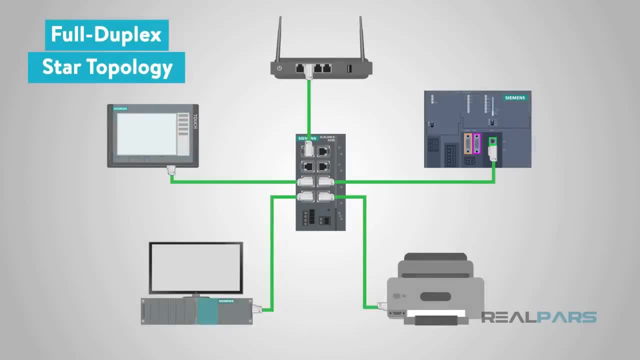 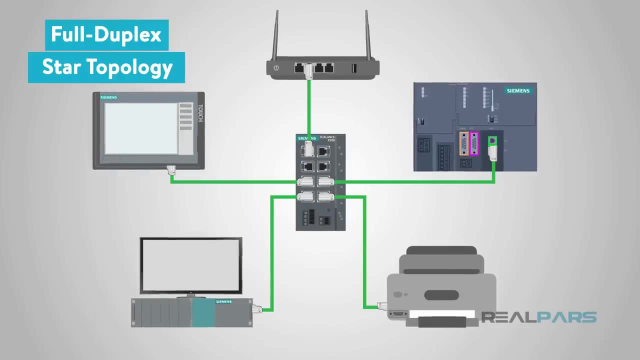 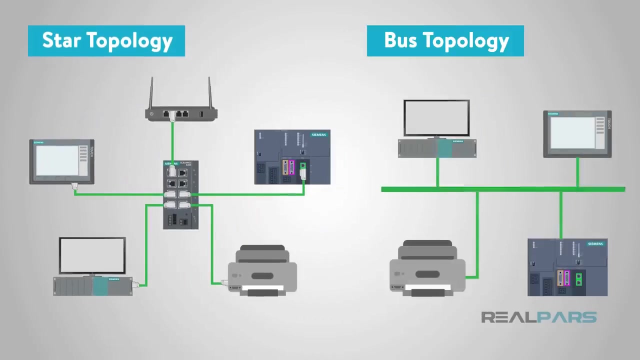 When you use the faster Ethernets in full duplex modes and incorporate switches, then you are utilizing a star topology between the switch ports and the devices. This allows for more direct transmission paths and fewer collisions as compared to a bus topology where all devices share the same paths. 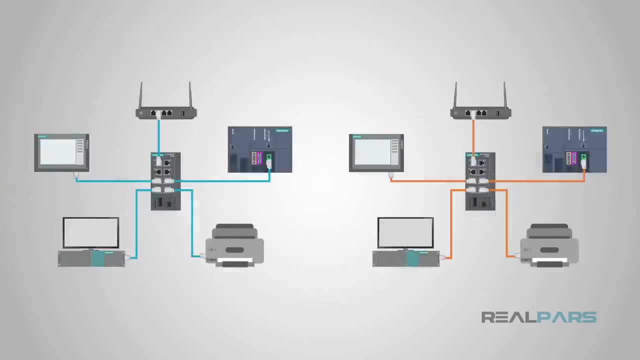 Ethernet capabilities are quickly changing with new technologies emerging every day. 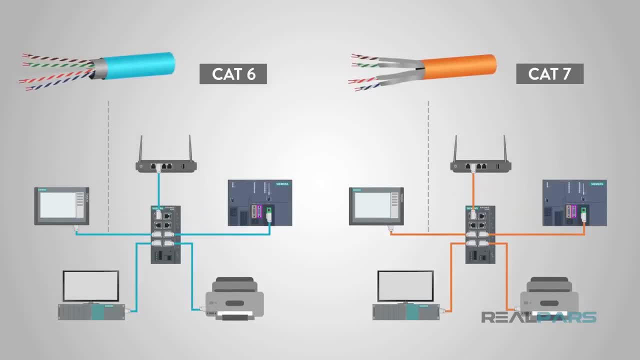 And while we are currently on the brink of successfully moving into speeds higher than the current 1 gigabits per second 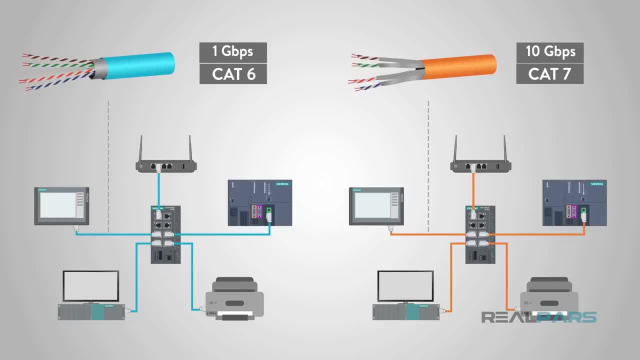 with 10 gigabits per second emerging over the last few years, these new Ethernet technologies will be costly. 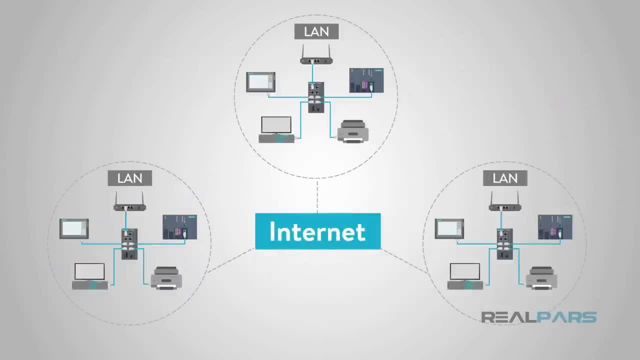 Also, your possibilities for the information world can seem endless when you connect this Ethernet local area network to the Internet to create a very large WAN, or wide area network. 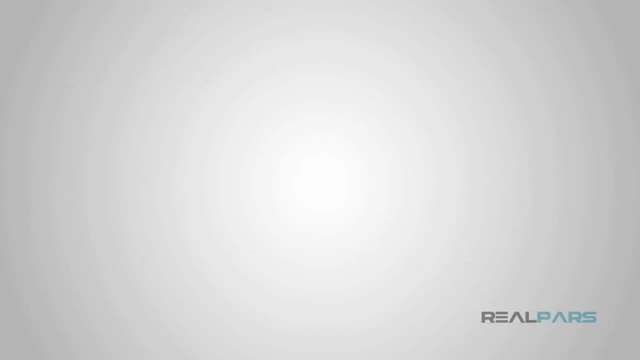 But that's a story for another day. All in all, Ethernet is popular because it strikes a good balance between speed, cost, and ease of installation. These benefits, combined with other features, combine with wide acceptance in the computer marketplace and the ability to support virtually all popular network protocols. 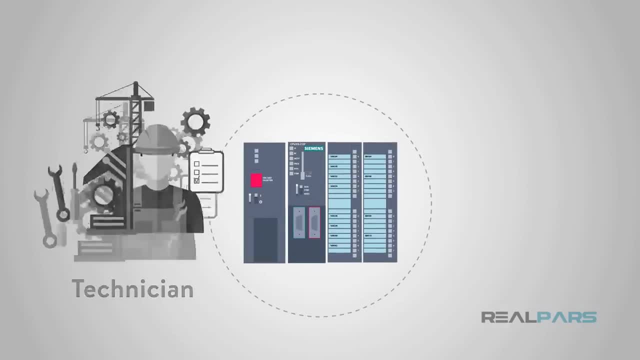 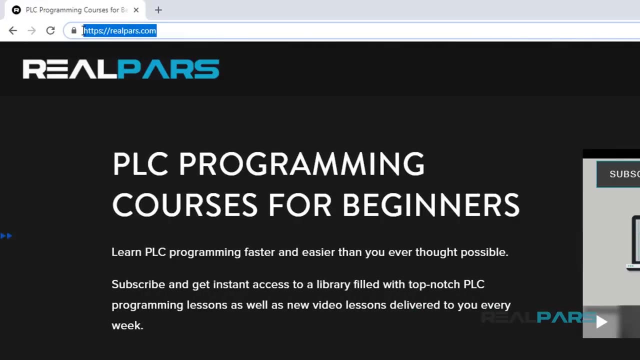 Want to learn PLC programming in an easy to understand format and take your career to the next level? Head on over to realpars.com 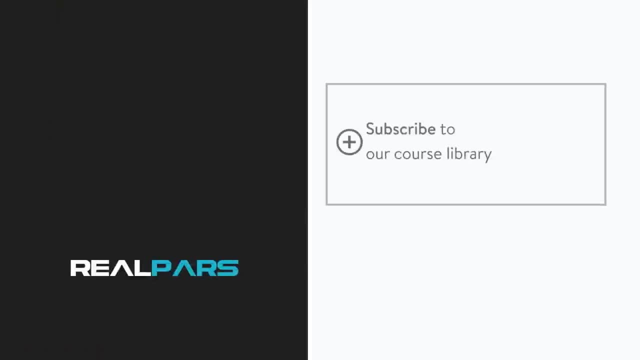 For more information, visit realpars.com.